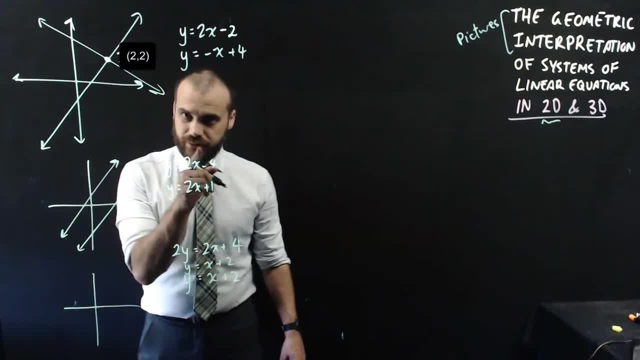 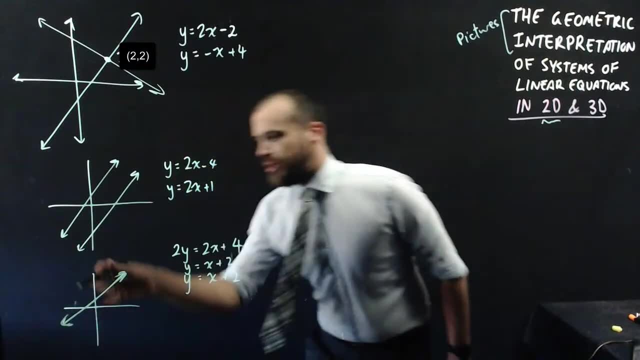 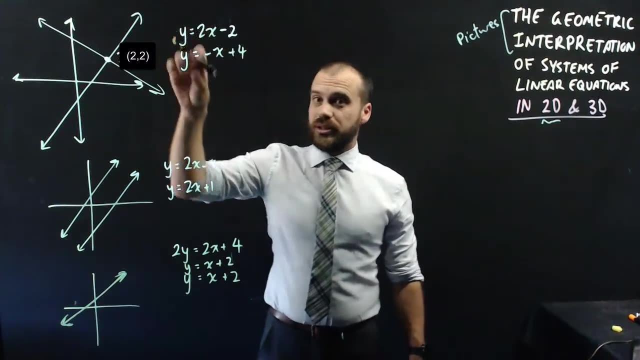 this line is the same as this line. so if I draw them, there's the first line but then the second line, I would need to draw right over the top again. There are two lines there. Okay, in conclusion, the geometric interpretation of systems of two linear equations in two dimensions can result in three. 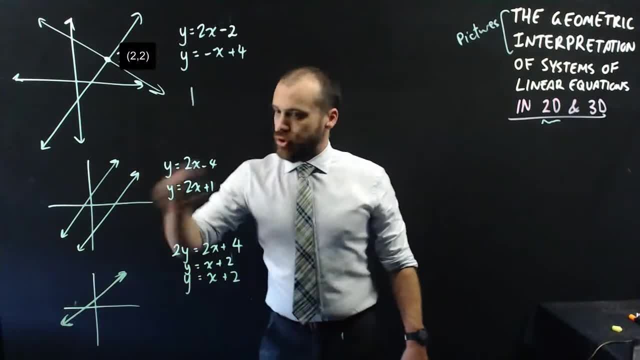 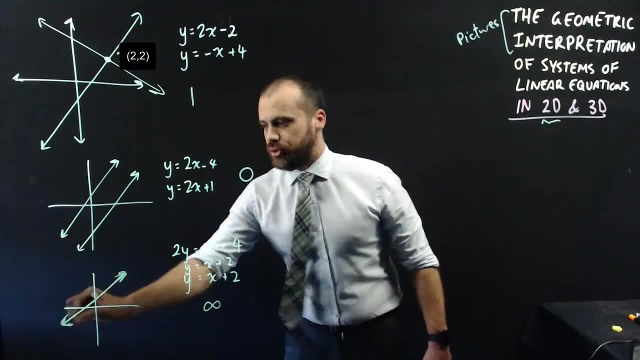 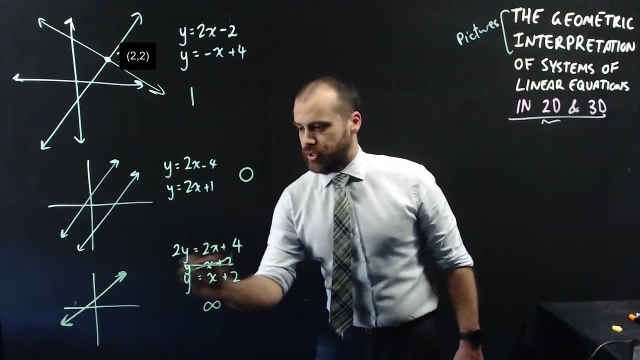 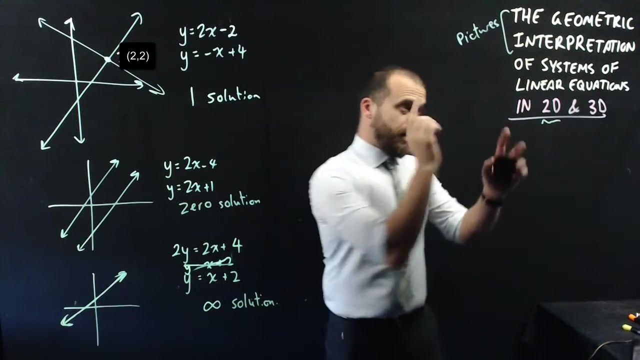 different things: One solution, no solutions or infinity solutions, because every single point along those two lines that are identical is a solution to that system Of linear equations. just right, that system of linear equations. So that's stuff you already know. It's not really what we're here to talk about. This 3D thing is what we're here to talk. 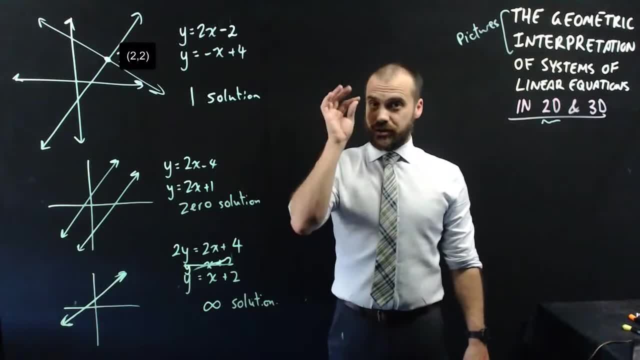 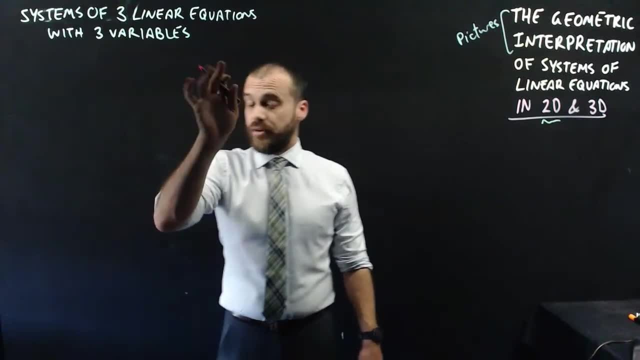 about, and this is where you're really going to have to start thinking, because it's hard to visualize, but luckily I've brought some props, So it's time to start talking about systems of three linear equations with three variables. So that's going to look something like this here. So those are all. 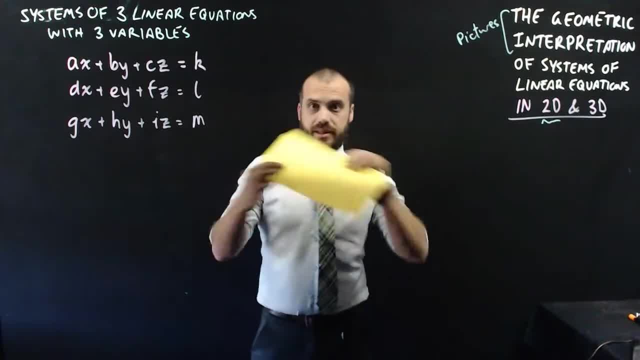 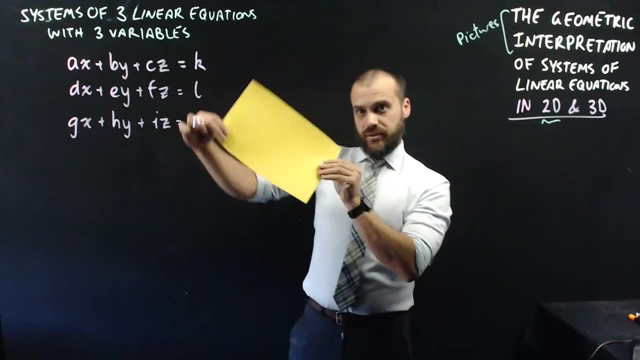 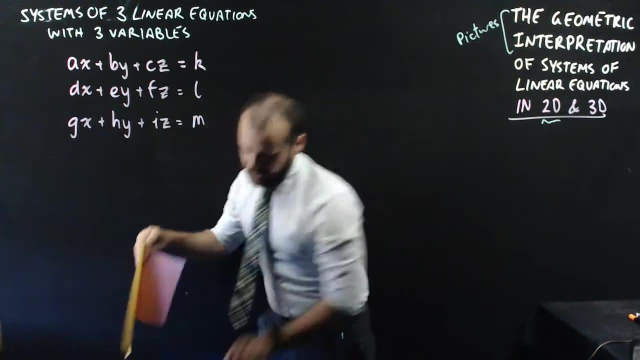 equations of planes right where a, b, c and k are all numbers and these are our variables. So this first plane might look a little bit like that on that angle, and then we've got another plane which might look a little bit like that, and then we've got another third plane that might look a slightly different. 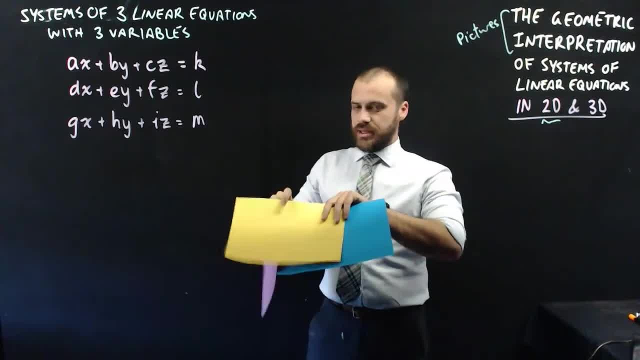 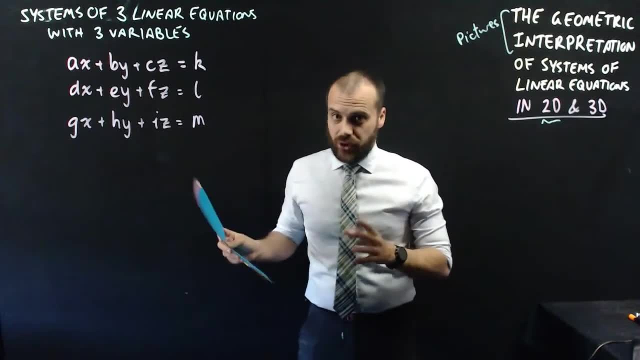 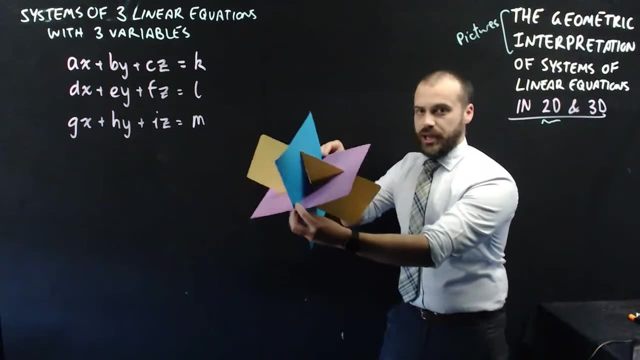 way and we're wondering how do these three planes interact with each other? So there are a variety of options, more than three options, like our lines had. Let's go through each of them in turn. Here's my first option. I have three planes here. They could be on any kind of 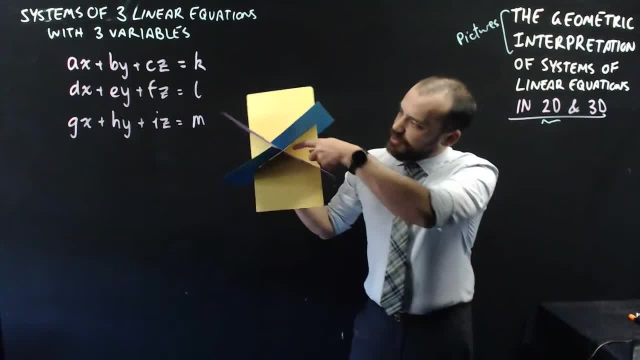 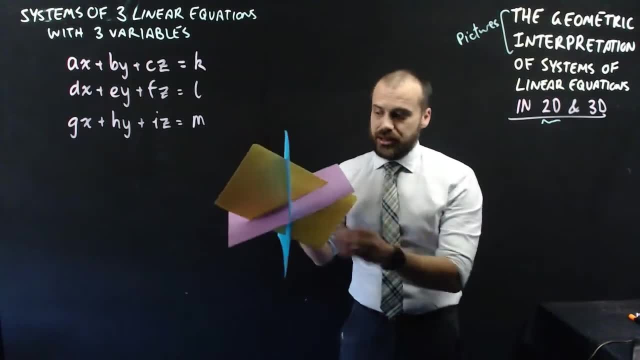 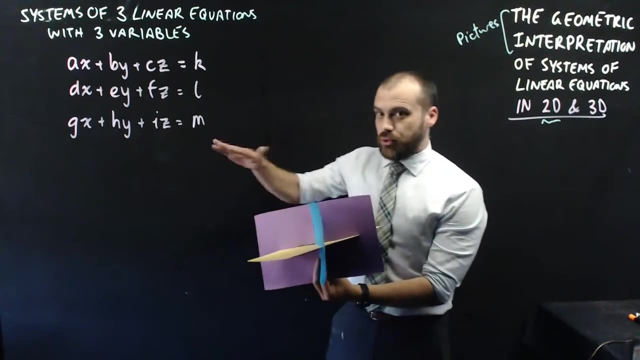 angle. but the important thing to note is there's this little tiny bit in there where they meet. These three planes meet at a single point there. Now you see this happen all the time. The floor of a room, one wall of the room and another wall of a room are three planes. 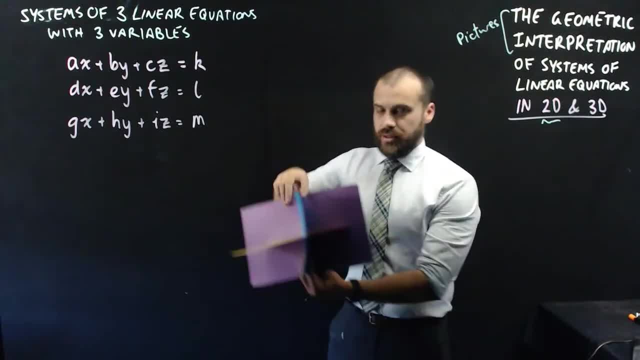 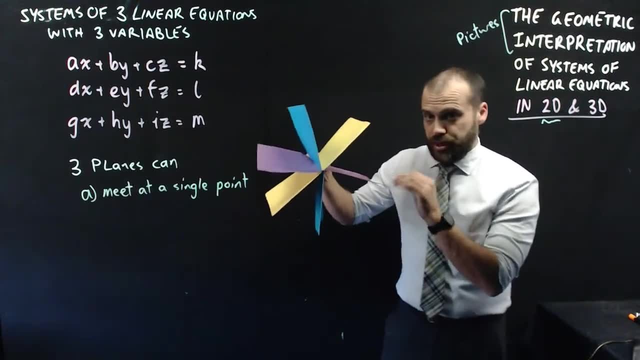 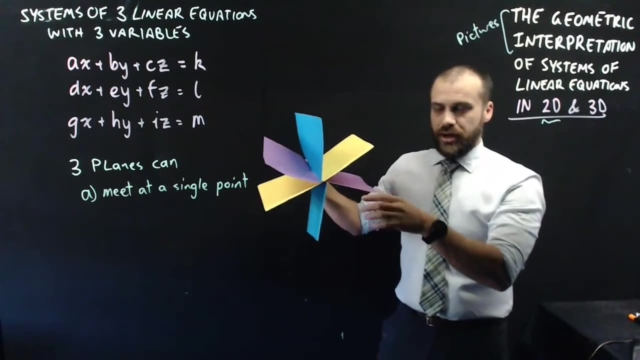 And they all meet at a single point. This is doing something similar. It's on a bit of a different angle, but same deal. Here's my second option. Now I've got three planes here and they've been placed through each other. They're meeting along a line, So these three planes aren't meeting at a single. 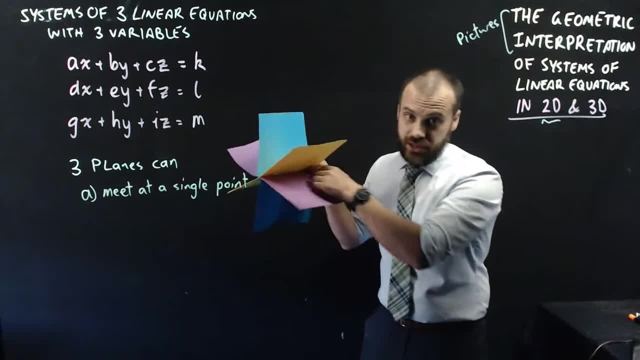 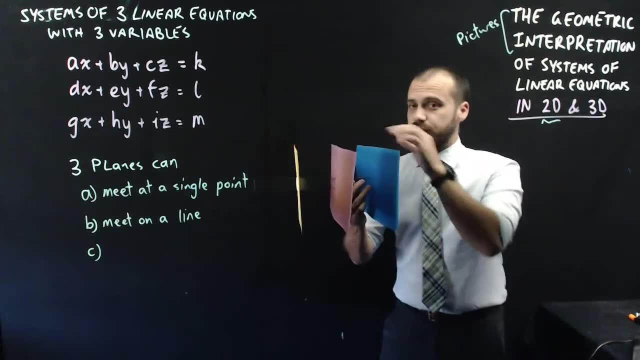 point. Instead, we can come up with a vector equation or a Cartesian equation for the line on which they meet. This one was fun to build, All right. So we have three planes here that all share the same normal. The ruler is the normal, Which means: 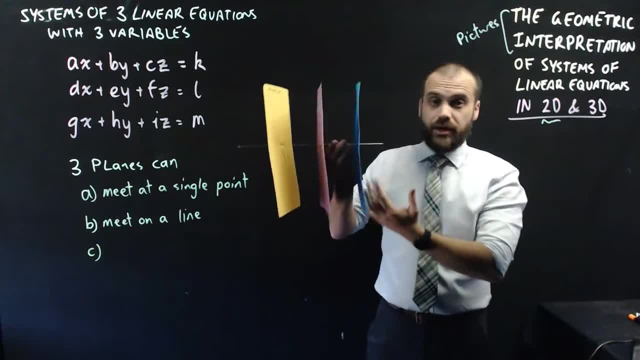 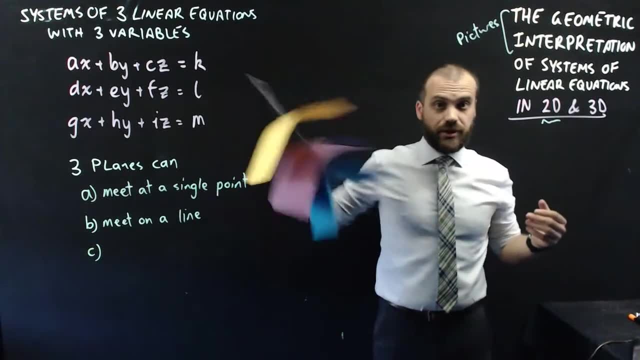 that they're all parallel to each other, Which means they will never meet. You can think of them as like floors in a building. That's probably a good way to think about it. But these three planes, they're never going to meet. We can end up in a sort of rocks is paper situation, where blue and 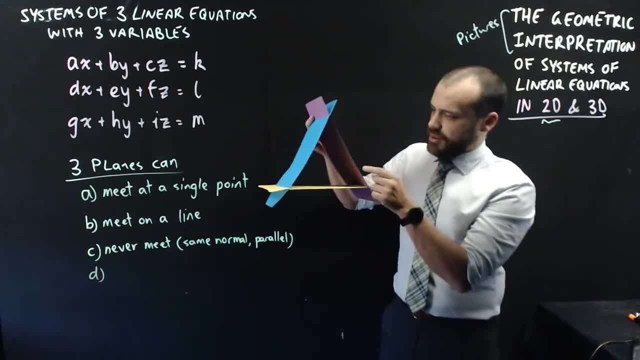 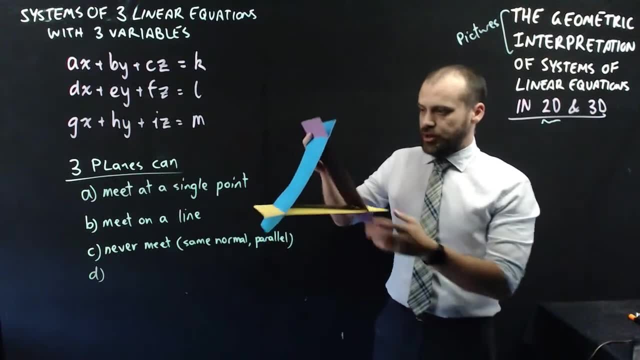 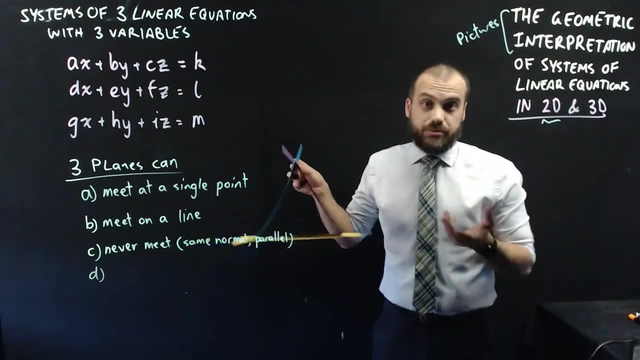 purple meet, Yellow and blue meet, Yellow and purple meet, But they have no common point of intersection, No common line of intersection. So this is another interesting way that three planes can not meet in this instance. You can also end up in weird situations like this, where you 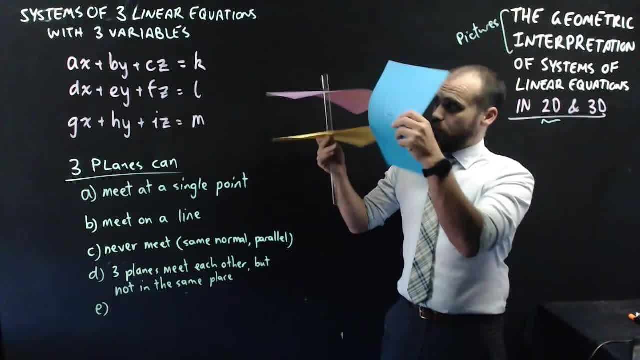 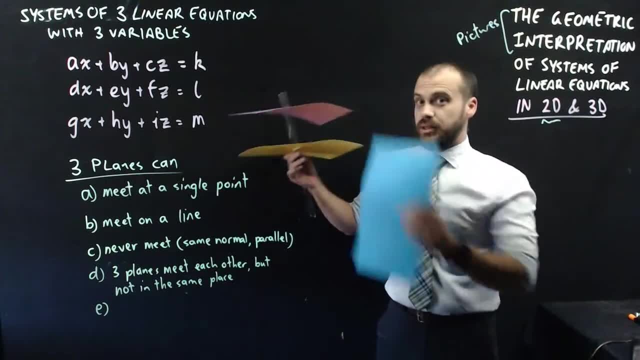 have two parallel ones- They share the same normal- And then one that cuts through the middle of those, So two that never meet and one that meets both of them. That's another option for our geometric interpretation And finally we get to this. 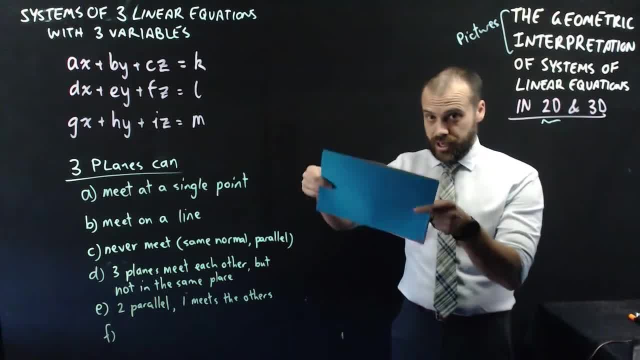 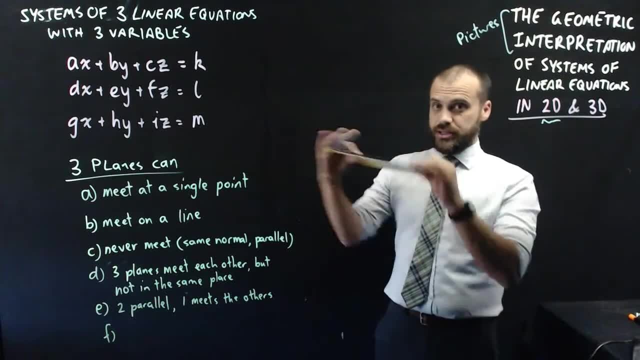 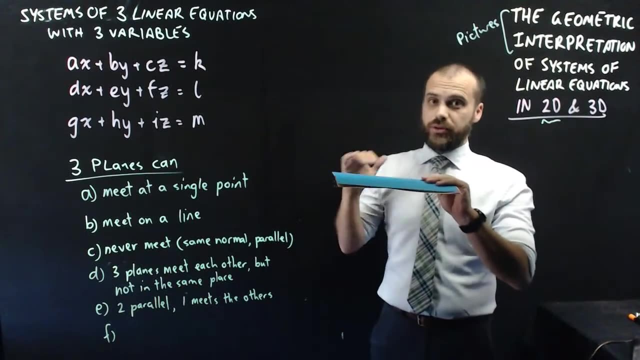 Three identical planes. So you'll remember that we had two identical lines when we were talking in 2D. We can have three identical planes as well. They are meeting at an infinite number of points. Every single point on the plane is a common point for all three of these, Or as a solution to the 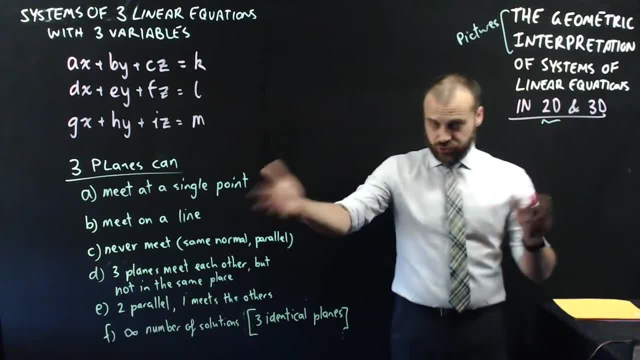 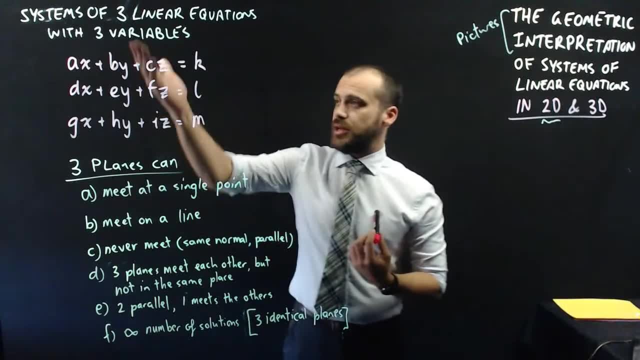 system of linear equations. Now you can do your best to draw these in your notes. Good luck with that. Now the three planes meet. Let's start off with the battery filter. So they're standing in front of the other plane. You can see that they meet. 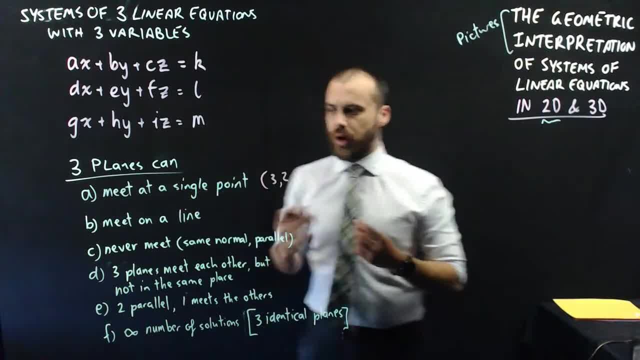 Everything is collectorQUI. Sloan looks like You can see that neverMUMBERETRITOS is a smaller button. You can see that they meet on a little obliged horizontal bar If you take a look at the UP and G as if, as in WALNUTPAY monitor. 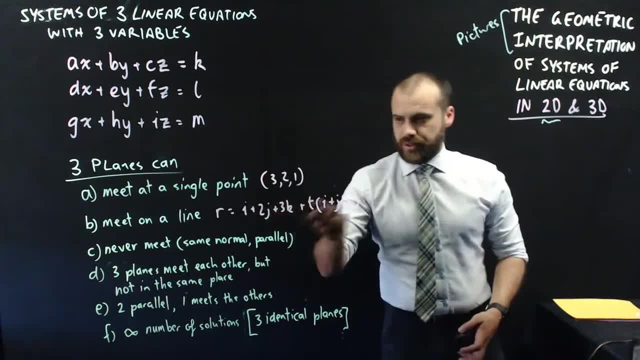 The battery is too well centered and there's no power to the length of the batteryiza. if there's no power to the length of the batteryiza, You can see in that way that the battery is 100 degrees. So from the bottom you have a counterpoint that like so.